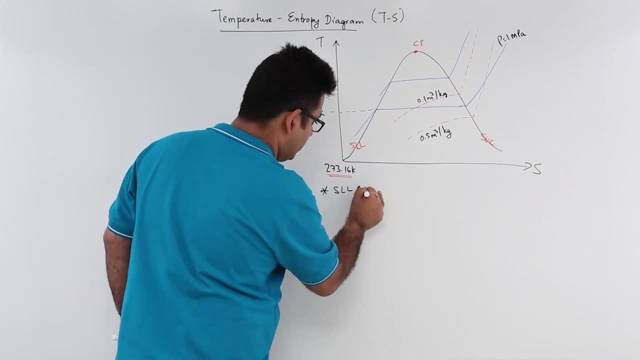 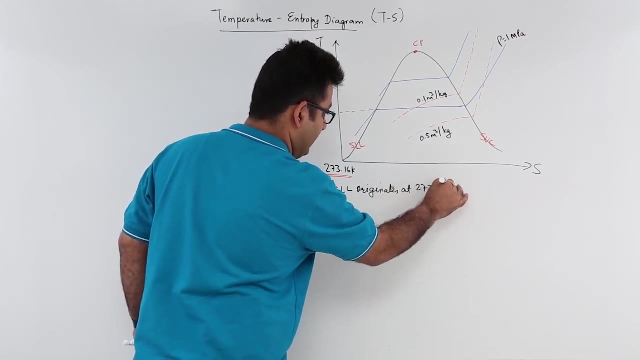 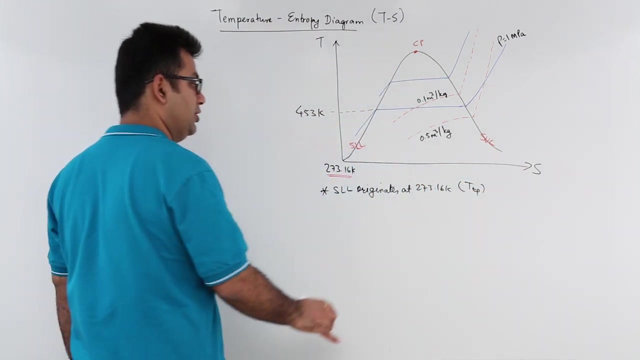 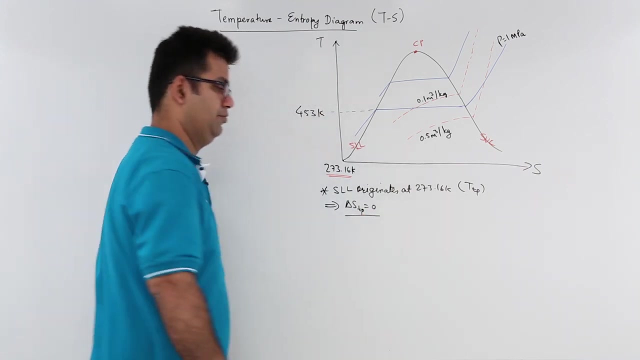 So your saturated liquid line originates at, at, at, at, at, at 273.16 Kelvin, and that is the triple point temperature for water, Isn't it? So this means that delta S for triple point is zero. Okay, Now there are two lines shown in blue color. 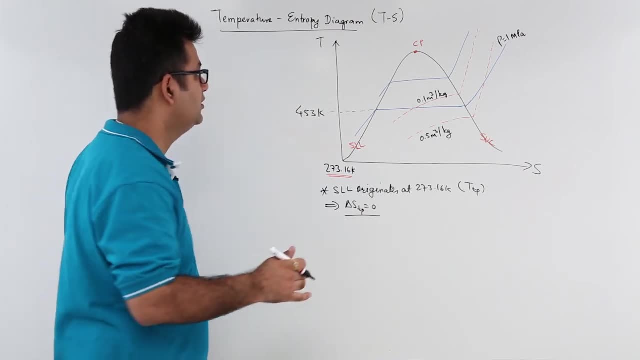 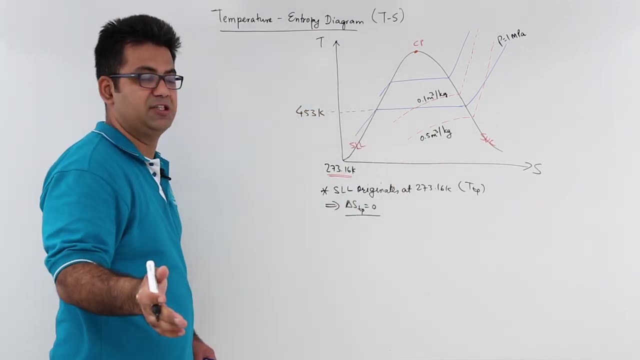 So these blue colored lines, they show two kind of things. Okay, So if you, before I go on to that, let's look at the regions you have in this diagram. So this SLL, SVL, it is dividing this whole graph into three regions. 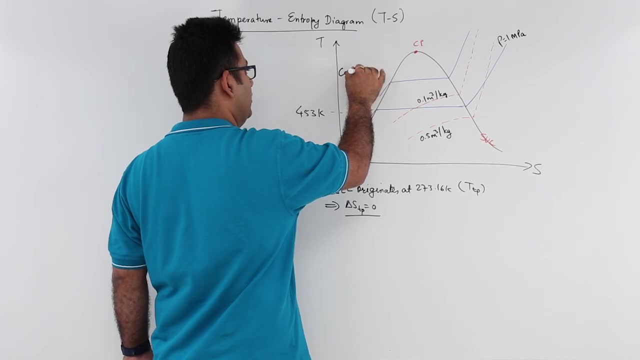 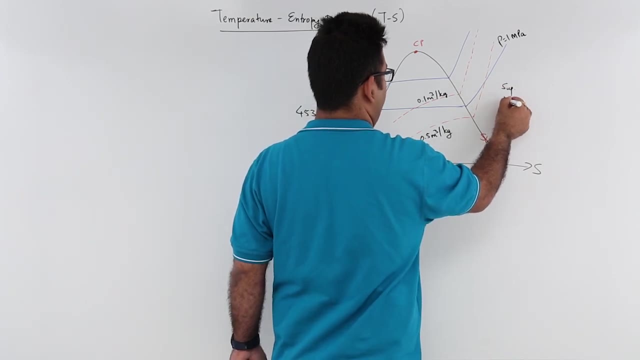 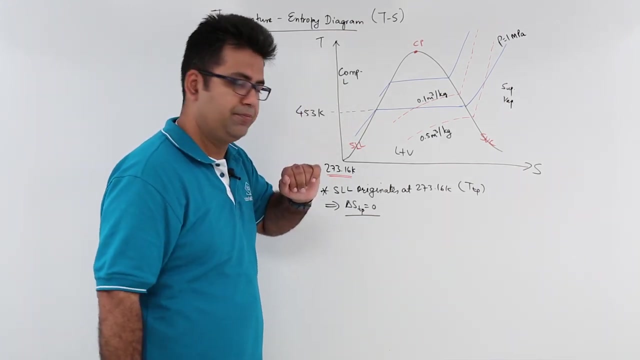 We all know that this is the compressed liquid or the sub cooled liquid, This is the liquid plus vapor region and this is the superheated vapor. Okay, Now in the compressed liquid region, this blue colored line, this slant line, okay, is the constant pressure line. 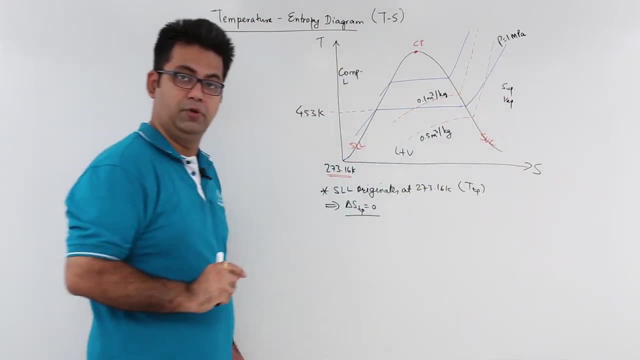 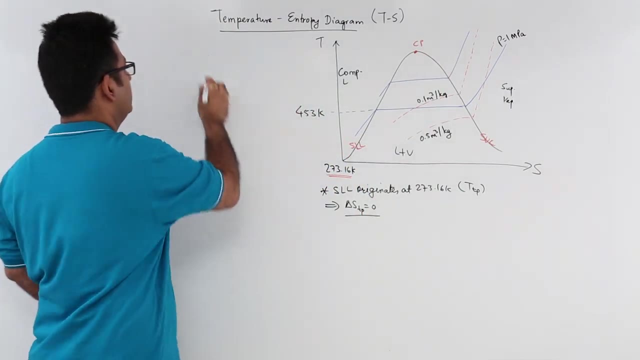 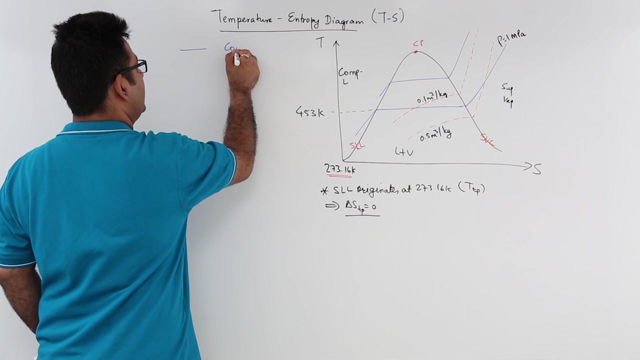 You can see this, Okay, So this is 1 MPa pressure and this would be higher than 1 MPa. So this blue colored line, if I draw it, this is a constant pressure line. So this is an isobar. 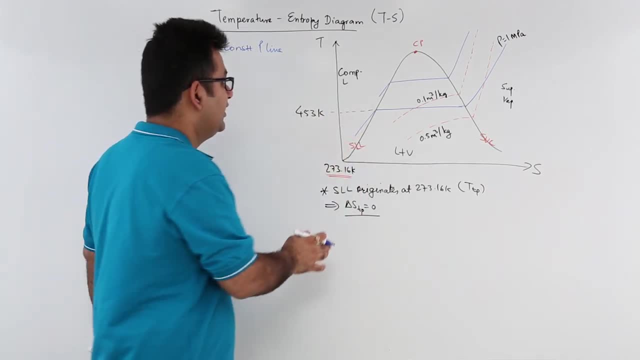 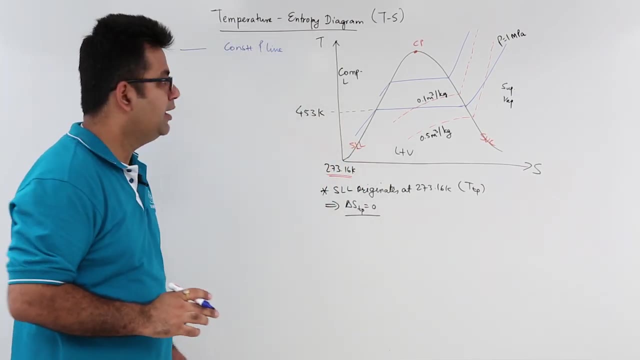 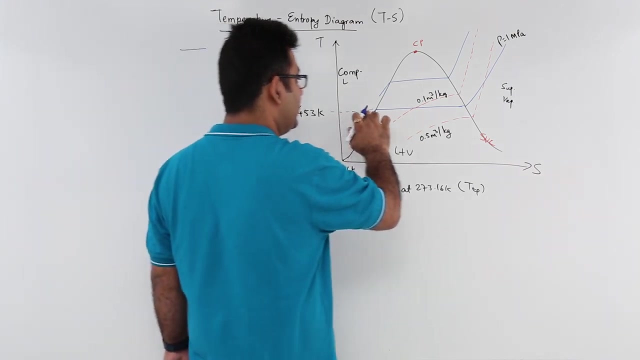 Okay Now, in the compressed liquid region the constant pressure line is almost the same. The saturated liquid line is almost coinciding with the saturated liquid line. Okay Now, when this constant pressure line comes into the liquid plus vapor wet region, it coincides or it becomes parallel to the isotherm. 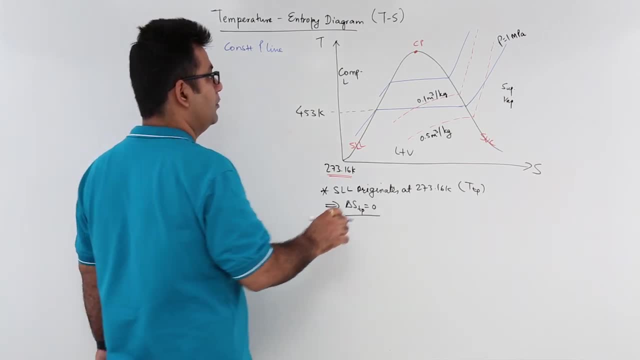 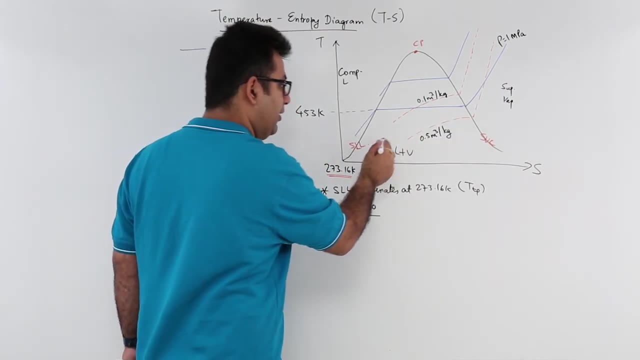 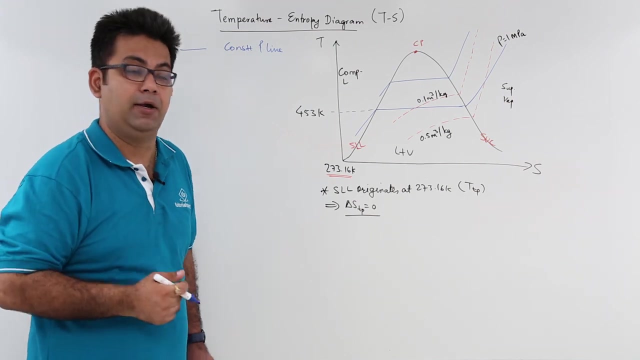 That is the constant temperature lines. Okay, Because this line is also constant temperature line, and in the liquid plus region, the constant temperature line and the constant pressure line, they become parallel to each other And then it, you know, has an upward trend.